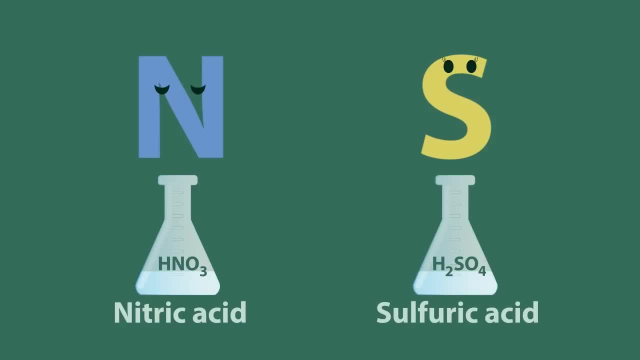 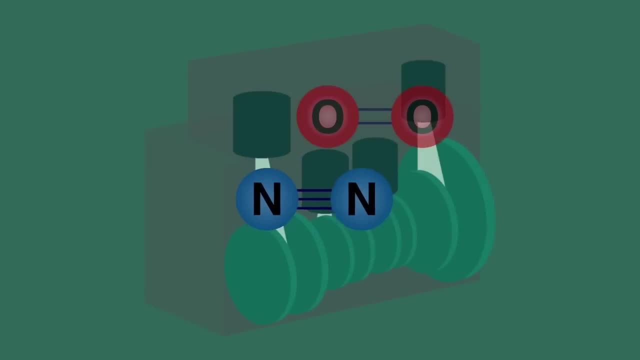 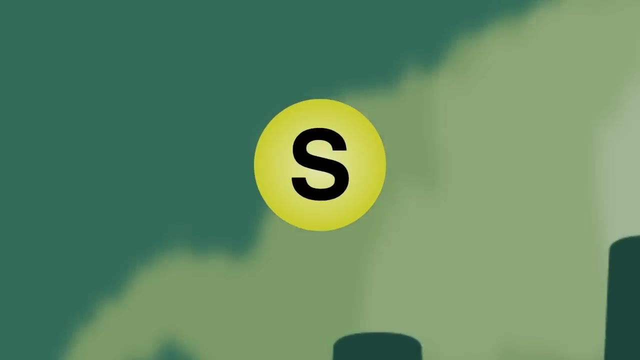 nitric acid and the sulfur. in the sulfuric acid, Pause and think. Well, the nitrogen came from the combination of atmospheric nitrogen and oxygen in the cylinders of motor vehicles. and the sulfur when fossil fuels containing sulfur are burnt, particularly in our power stations. Let's look. 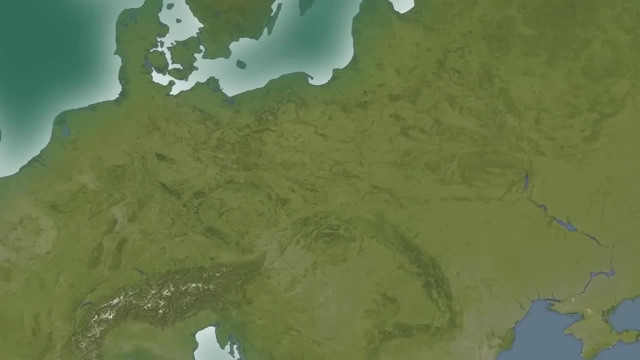 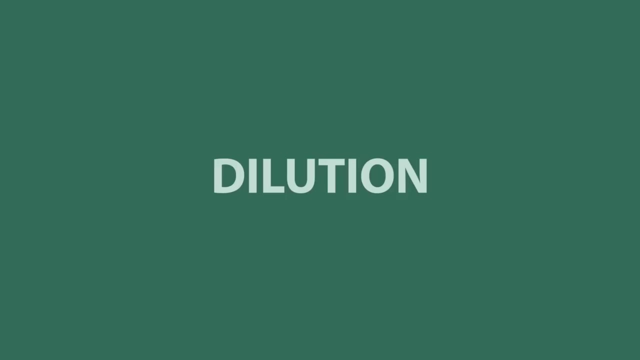 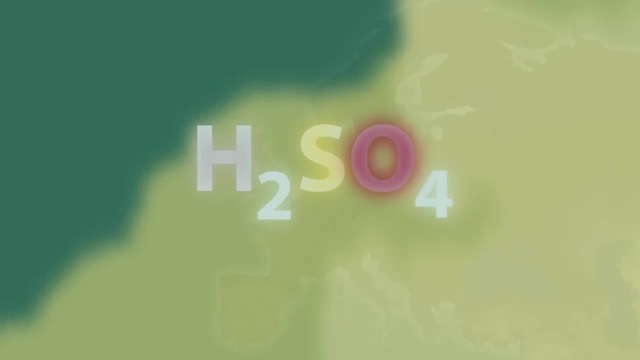 at power stations in Europe. For many years, these stations have been using tall chimneys to disperse the sulfur dioxide far away, thinking that dilution was the solution to pollution. However, the acid did not get diluted, but instead was carried in the wind to Scandinavia, where it fell into Swedish. lakes. Originally, people tried to neutralize the acidity by adding limestone to the lakes. This was partly successful. For example, salmon returned to some polluted rivers in Wales after the acidified lakes from which the rivers flowed were treated with lime over a number of years. A much better. 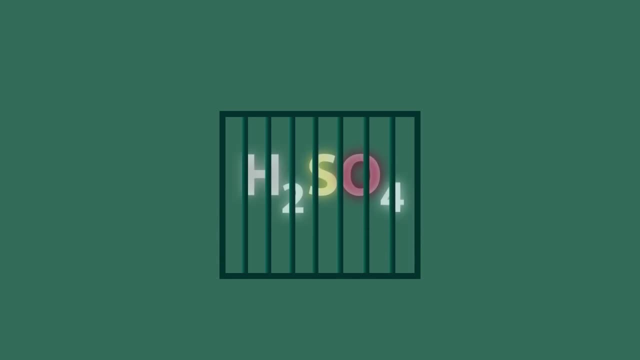 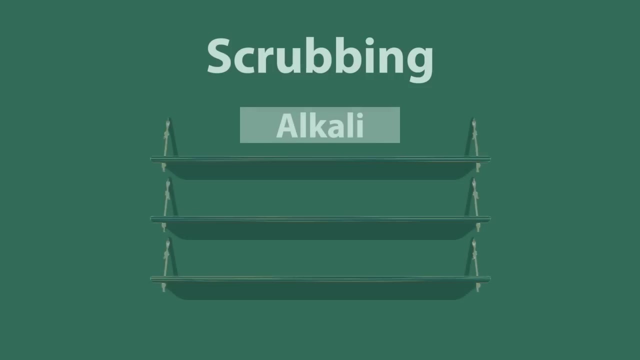 method is to trap the acid before it reaches the atmosphere in a process called scrubbing. The kind of scrubber we need in this case is an alkali to react with the sulfur dioxide. so either seawater, which contains a little bit of sodium carbonate, or lye, which contains a highly acidic acid, but also arguably the most affordable way to react with the sulfur dioxide is to add limestone. so either seawater, which contains a little bit of sodium carbonate, or lye or leucine, which contains a little bit of sulfur dioxide, or the other way round, we can use the most effective method, and this is known as the lips of the sea, but you don't have to. 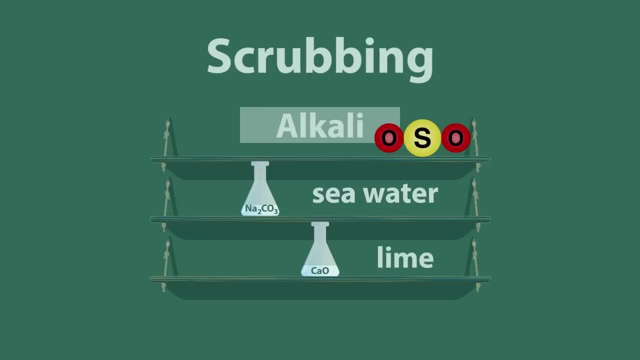 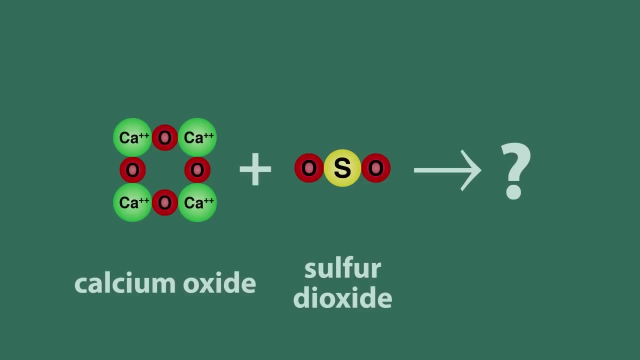 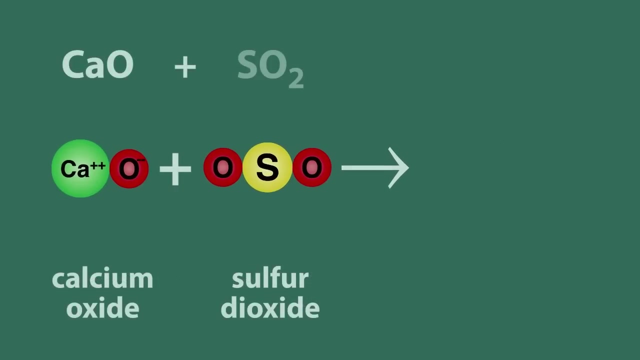 lime calcium oxide is used, Can you think what reaction will occur with calcium oxide, a basic oxide, and sulphur dioxide, an acidic oxide? Calcium oxide plus sulphur dioxide makes calcium sulphite, that's CaSO3.. The sulphite can be reacted with oxygen to make gypsum, calcium sulphate, CaSO4,. 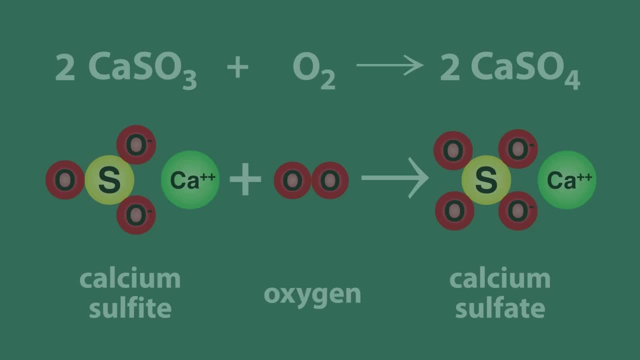 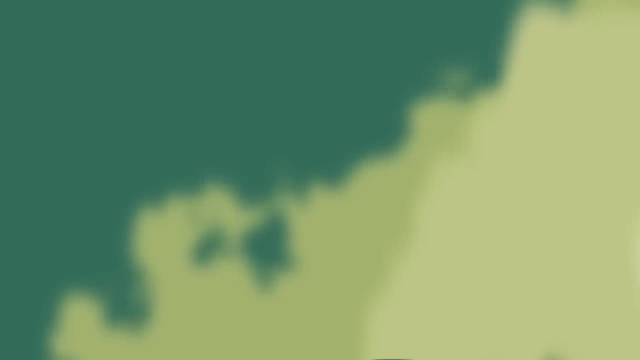 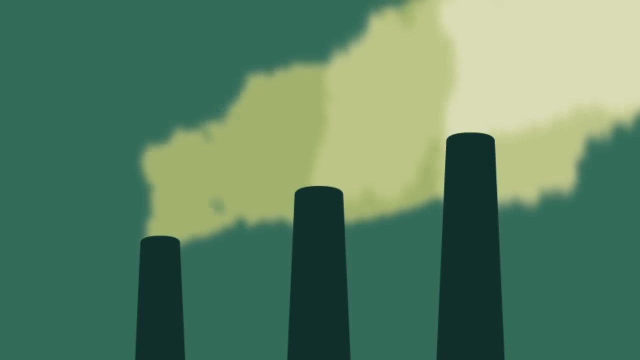 which is the main ingredient of wall plaster. These scrubbers have greatly reduced our sulphur emissions and given many countries much cleaner air, but it does reduce the efficiency of the power station, maybe by as much as 10%, thus increasing the cost of the electricity In oil refineries. sulphur is removed. 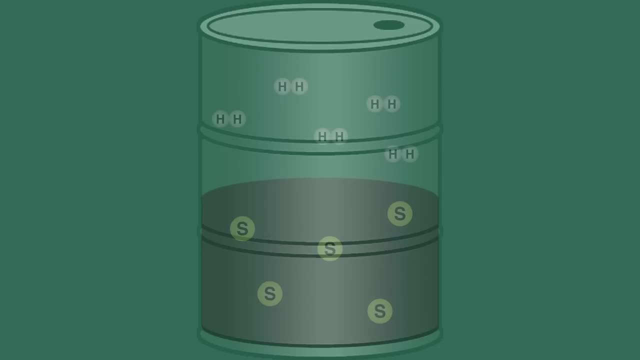 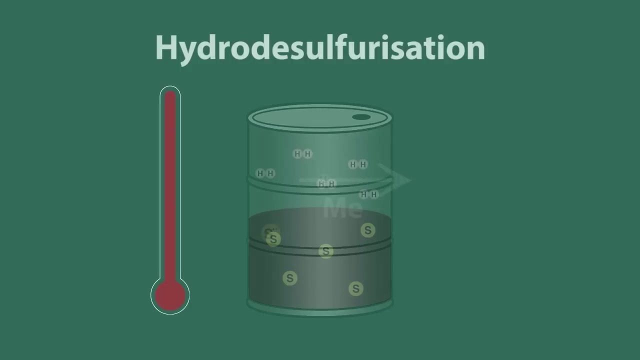 from crude oil by reactants. This reaction, known in industry as hydrode-sulphurisation, takes place at high temperature with a metal catalyst to produce hydrogen sulfide- that bad egg smell and a very poisonous gas When this purified oil is refined.